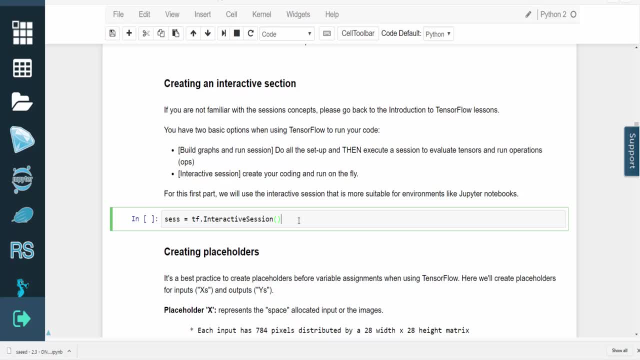 the graphs and then run the session, or we can use an interactive session in order to create code and run everything on the fly. Since the latter case is more suitable for a Jupyter Notebook environment, we'll use the interactive session. It's good practice to create placeholders in TensorFlow before variable assignment. 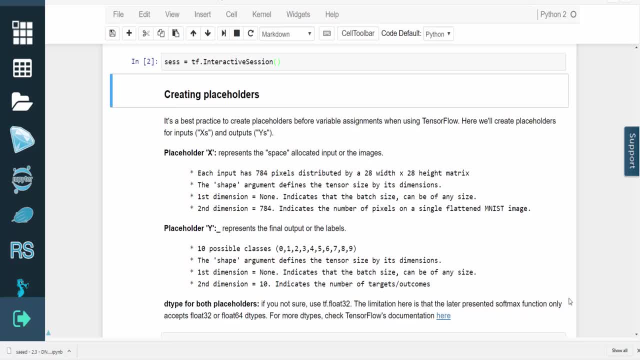 Placeholder x represents the space that will be allocated to the input, which is the set of handwritten digit images. Placeholder y represents the final output, which are the digit labels. You'll need to select a D-type for both of the placeholders and, if you're not sure, 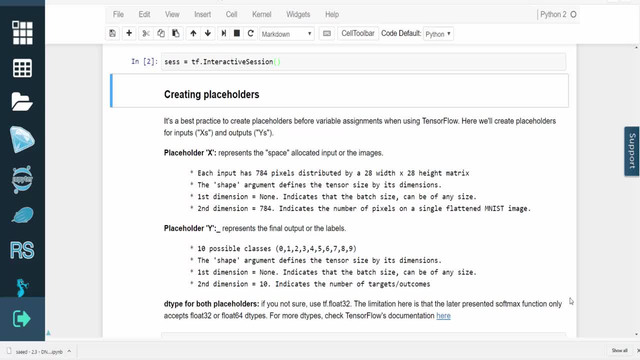 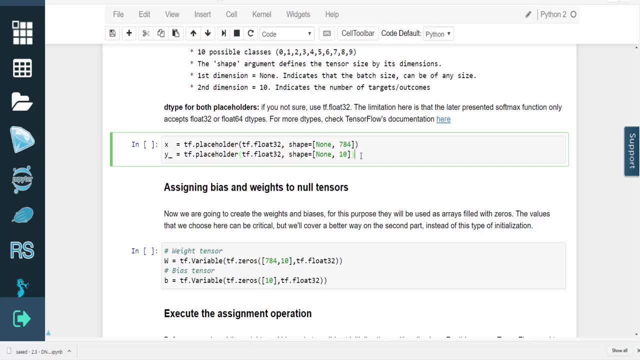 just use tffloat32.. It's worth noting that the softmax function, which we'll cover shortly, only accepts float32 and float64.. For more D-types you can check out TensorFlow's documentation here. Now we are going to create a multilayer perceptron for the MNIST database We're going to create. 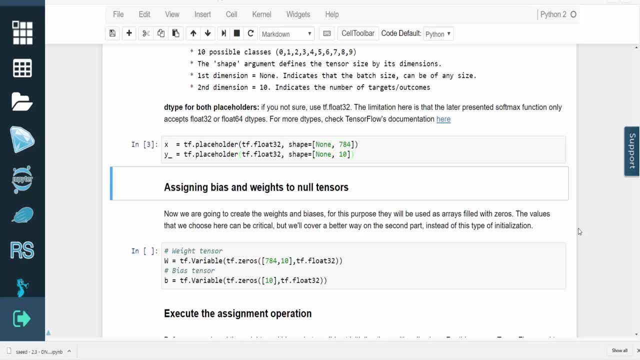 the weights and biases for our neural network. The initial choice of values is critical, but at this point we'll just use arrays filled with zeros. Before, we told TensorFlow that we assigned the weights and biases, but we didn't initialize them with null values. As a result, TensorFlow needs to initialize the variables that you 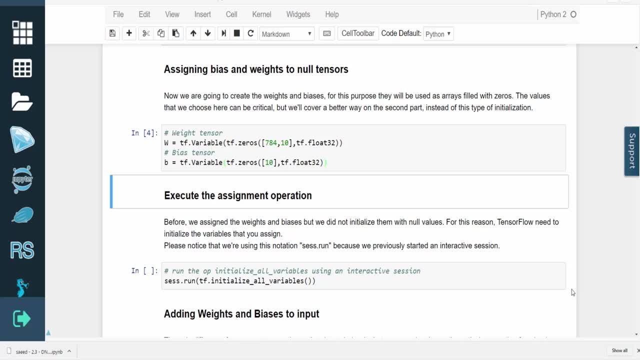 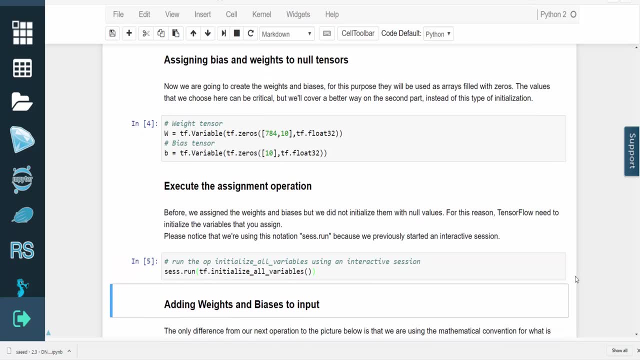 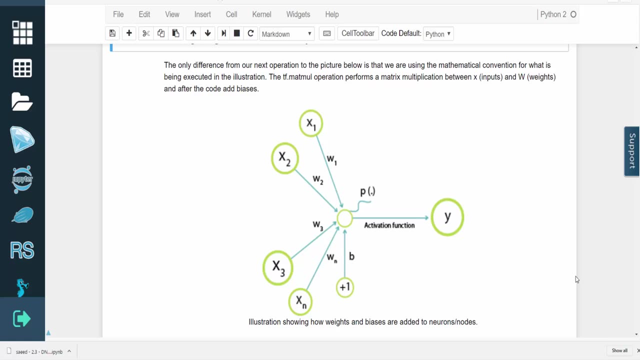 assign. Also note that we're using the notation sesrun, since we previously started in TensorFlow. The picture below shows how weights and biases are added to the neurons in a network. Our code performs this using the mathematical notation with matrices, The tfmatmul operation. 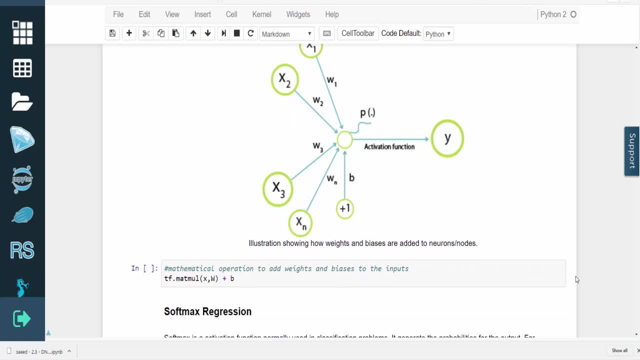 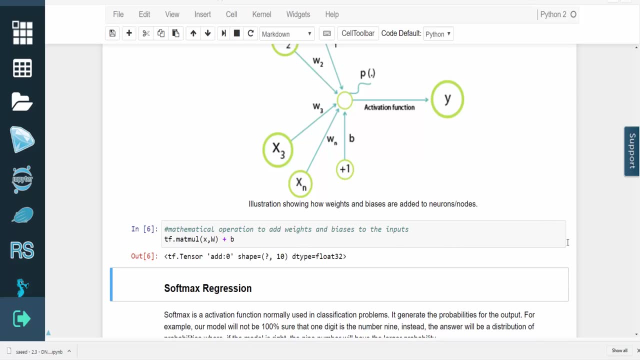 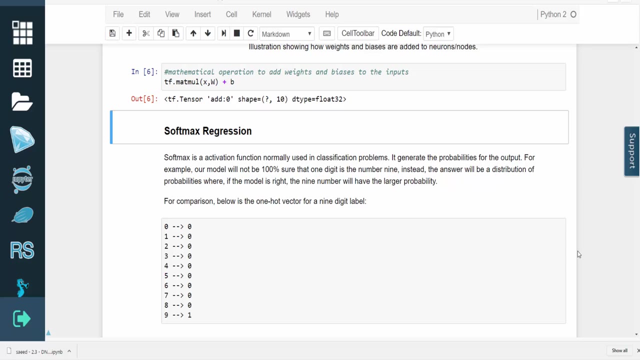 performs a matrix multiplication between x and w, which are the inputs and weights respectively. The code also adds on the bias values. The tfmatmul function is a popular activation function for classification problems. Rather than simply outputting a yes-no answer for its prediction, it will generate a probability. 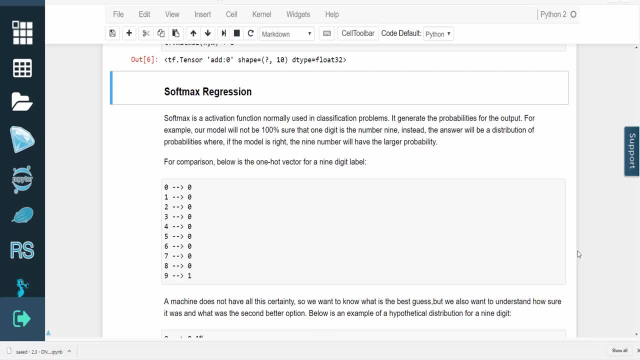 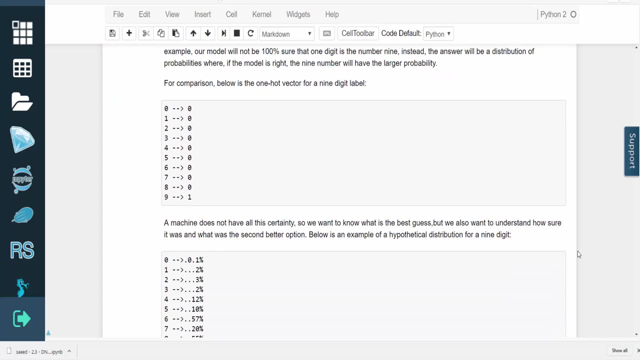 value for each potential output. The model will never be 100% certain of its answer, so this technique is useful for gauging the model's confidence for each potential answer. So, for example, the model might calculate that the digit 9 has the highest probability. Here you can see the one-hot vector representation.